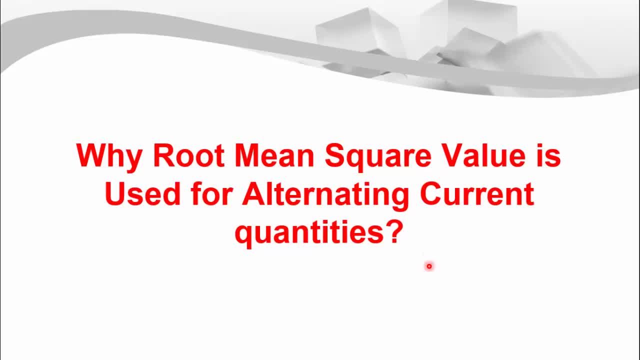 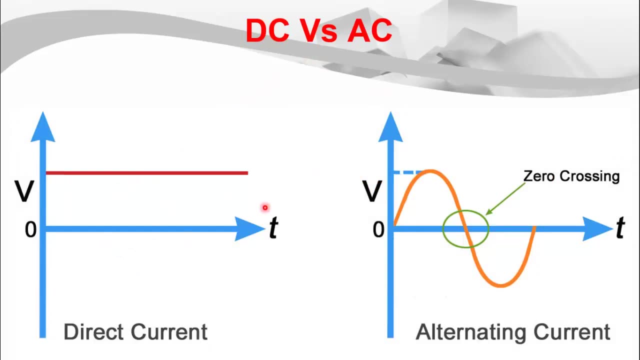 and at the end of this video we will see the significance of root mean square value for voltage and current. in order to answer this question, we'll start by seeing the difference between the direct current and the alternating current quantities. on my left you can see the DC voltage and DC quantity has a straight. 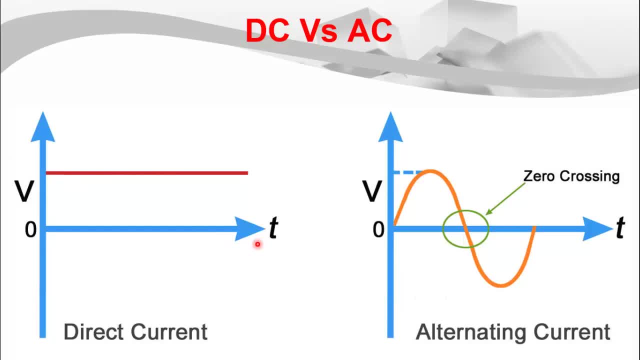 line with respect to the time. it means that its values never changes with the time. there might be small oscillations due to the result of disturbance, but the magnitude of the voltage or the current or any quantity will remain the same throughout the time, whereas in alternating current the value or the magnitude keeps changing with the. 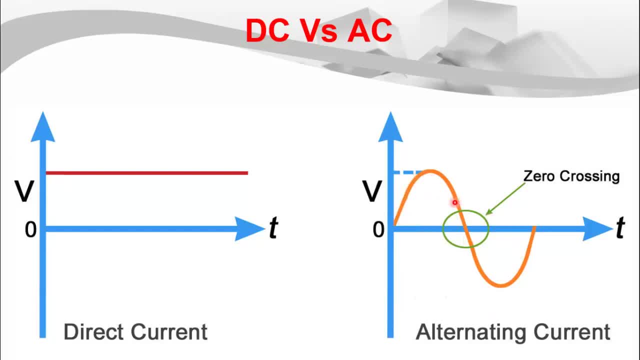 time. Here you can see a sine wave. normally a sine waveform is used for voltage and current quantities. so in half cycle it has the positive values and in other half cycle it has the same values, but with opposite direction. and there will always be a zero crossing between the half cycles. here we take a closer look. 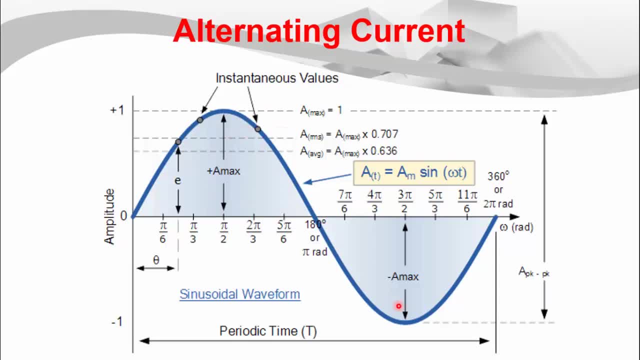 into the alternating current. alternating current waveform, as you can see here that a plus is the peak or the maximum value of this waveform and other than this, the magnitude of this waveform is changing with the time and you will have different values on different time, instant, in both the positive and the negative. 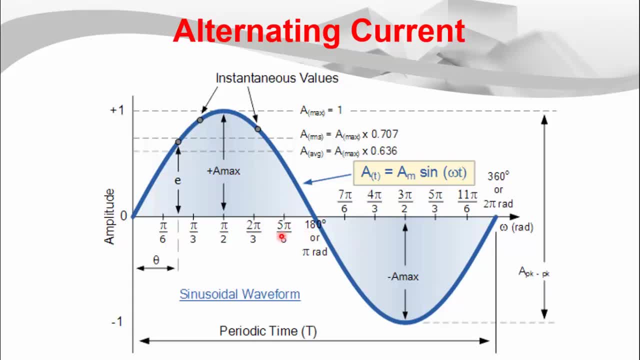 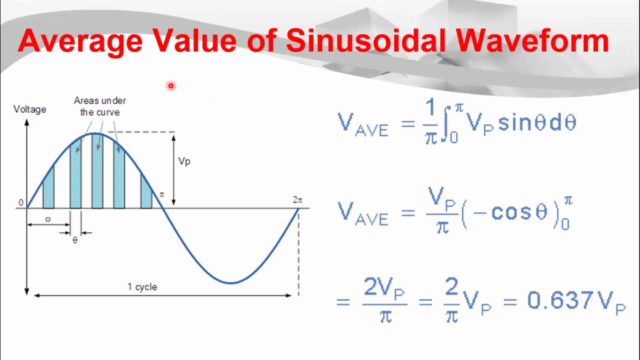 cycle. so whenever you have to tell the magnitude of the voltage or the current, you have to give a single value. you must have a mechanism to compute this whole waveform into a single value which indicates the magnitude of the complete waveform. we can have one mechanism to compute the average. 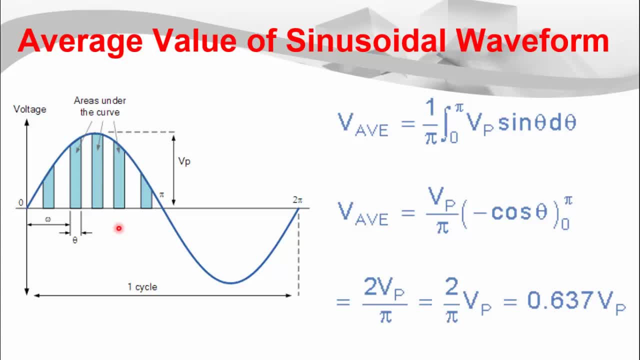 value of the sinusoidal waveform. so after knowing much about the AC waveform, we have learned that the complete cycle in which we have positive and the negative cycle have the exact same values but with opposite sign. so if we add all the values in the complete cycle, the 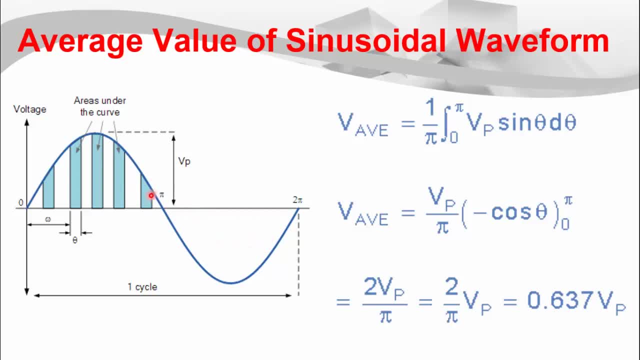 overall average value comes out to be 0. in that case, we only have to take the average value of half cycle, which comes out to be 0, 0.637 of the VP, and VP is the peak value. so here you have the single value, which is equivalent to 0.6. 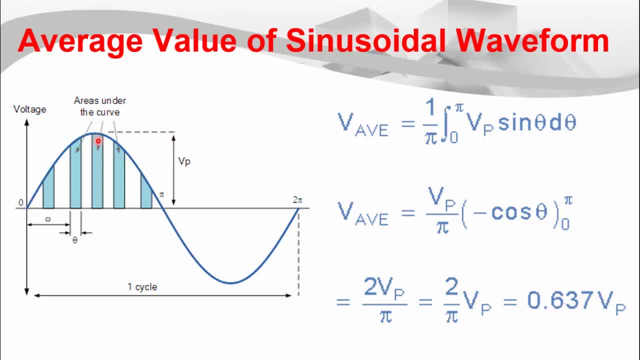 of the peak value, but this value represents only the half cycle but in actual we have full wave AC waveforms. therefore we cannot use the average value because the average value of the full waveform is 0- 0.637. so we need to find another mechanism that we give the exact picture or the exact quantity of 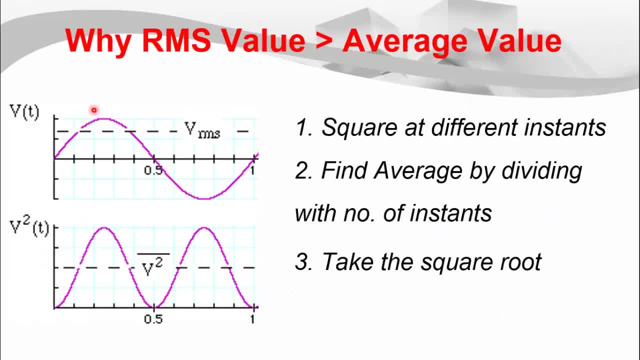 the AC waveform in a complete cycle. so let's suppose we have this waveform. the first step is to take the square of this waveform. in that case the waveform will have all the positive values in one complete cycle: 0.637. the next step is to take the magnitude at different instance while the amplitude is total, and then we are. 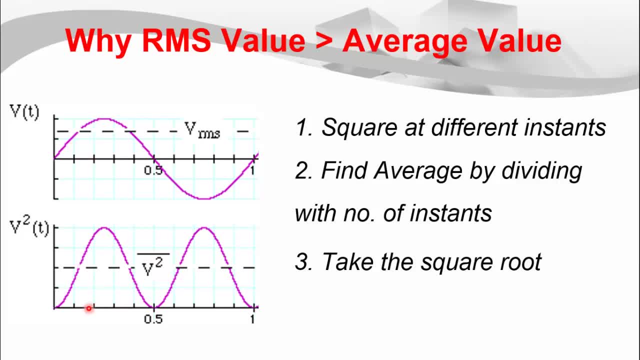 and then divide with the number of instance to get the average value. now we have already scaled this waveform, so in order to find the actual value, we need to take the square root in the last step to find out the actual value, which will be equal to the root mean square value. 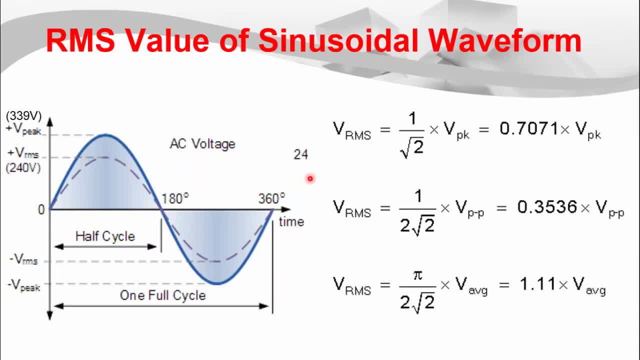 of this waveform and by following all the steps to find the vrms, the voltage, the root mean square value of the voltage comes out to be 0.707 of the peak voltage. so we, if we have the peak voltage equal to 339 volts, the root mean square value comes out to be 240 volts and this is the value. 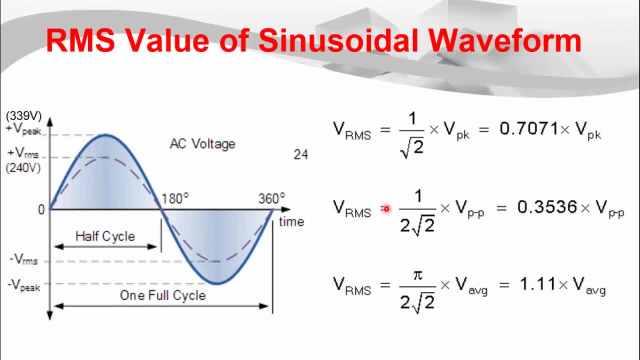 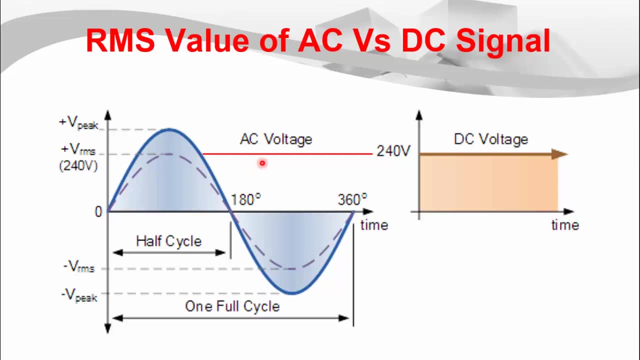 of the single phase voltage in most of the countries once we have the rms value, which represents the value of the complete sine wave. now i will tell the significance of this rms value. the rms value of the ac quantity is equivalent to the dc value. it means that 240 volt rms ac voltage is equal to 240 volt dc voltage.